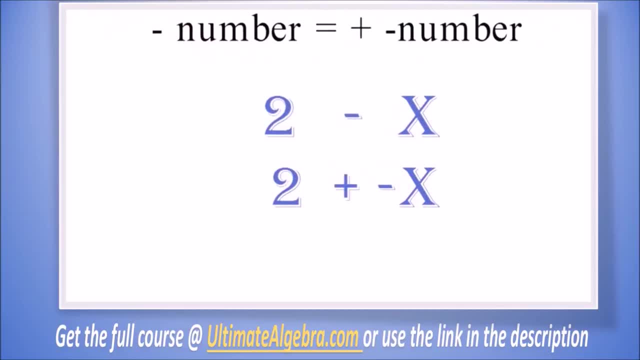 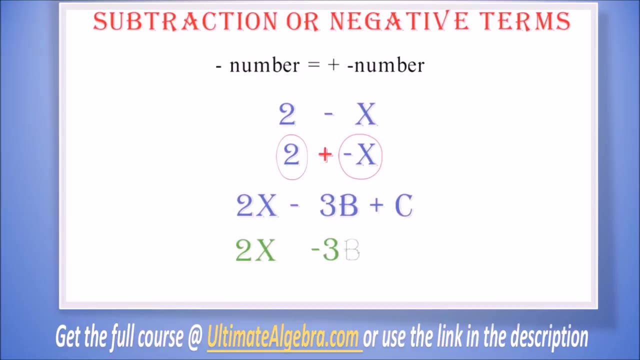 are separated by a plus sign. So we can still say that the 2 is one term and the minus x is another term, and they are separated by a plus sign. With this in mind, we can say that the terms in 2x minus 3b plus c are 2x negative 3b and. 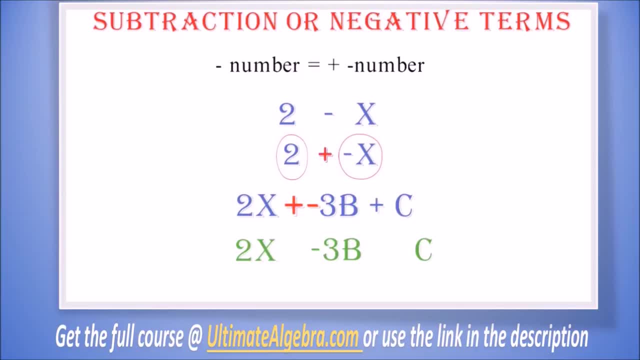 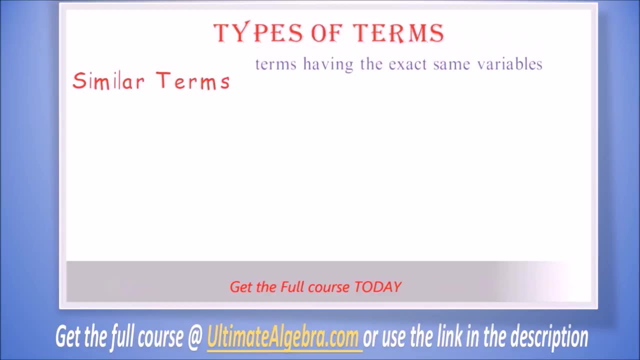 c, We change the minus to plus negative. Hope everything is clear up to this point. Types of Terms, Similar or like terms, are terms having the exact same variables. These variables must have the same exponents. Remember we said the variables are simply the letters. 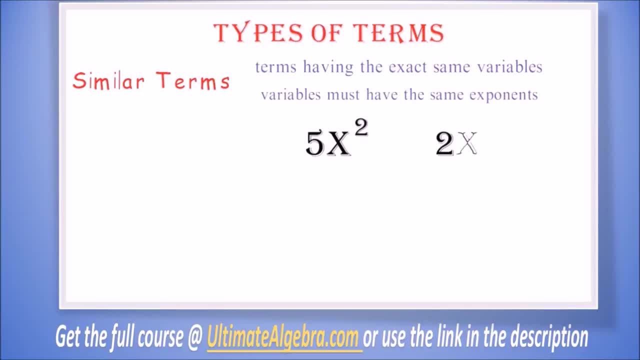 Example, When we look at 5x squared and 2x squared, we'll notice that both have the letter x and the x has the same exponent too, So we can say that the terms are similar. 2ab and 4ab are also similar terms because they both have the same variables or letters. 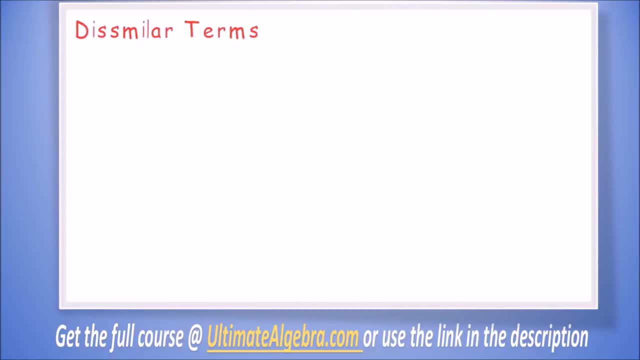 and those variables have the same exponents. Dissimilar terms are terms which differ in variables or exponents or both. Example: 3x squared and 4x cubed. Here both have the same variable x, but different exponents. One is squared and the other is cubed. 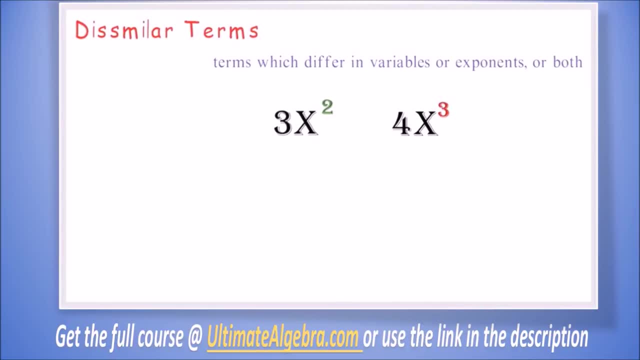 Though they have the same variable, because they have different exponents, we say they are dissimilar terms. Another example: 2cd and 4mb. Notice they have different letters, One is cd and the other mb, so they are dissimilar terms. 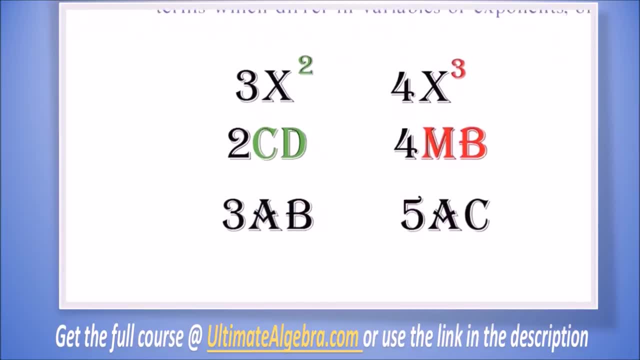 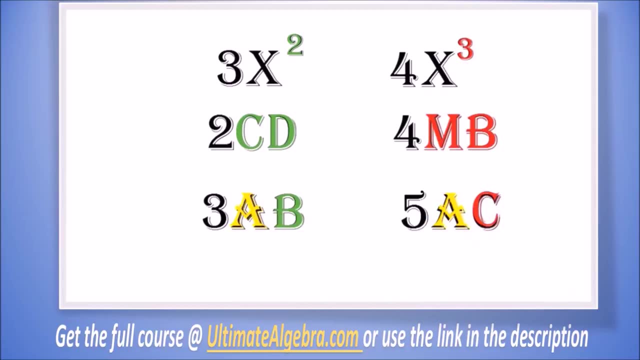 One more example: 3ab and 5ac. Now Here we see that they both have the variable a, but one is ab and the other is ac. They are still dissimilar terms. All the letters must be exactly the same. 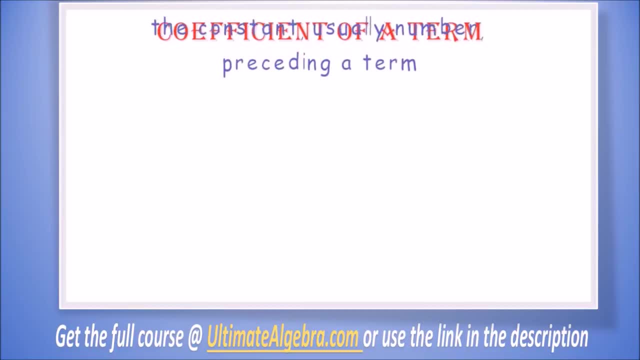 Coefficient of a term. Now let's look at the coefficient of a term. The coefficient of a term is the constant, usually number, preceding a term. So far we've been looking at the variables. Now let's look at the number. If we look at a term 3x, the coefficient is 3.. 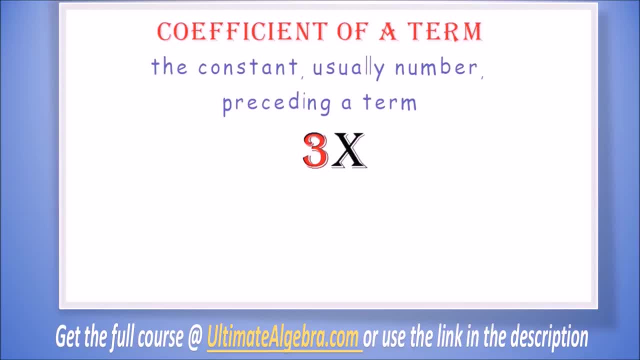 3 is the constant preceding the term. In algebra it is possible to have a term which consists of only letter. Example xy. In a case like this, where there are only letters, the coefficient is 1.. So xy is the same as 1xy.